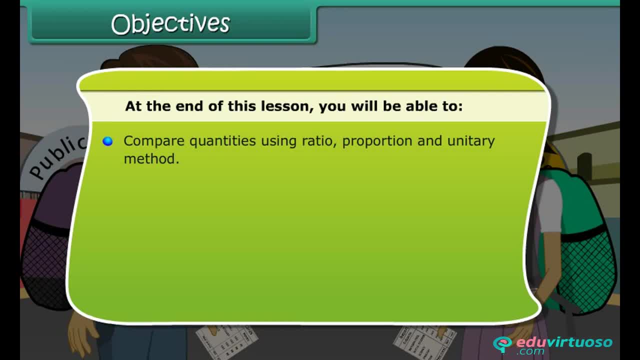 Compare quantities using ratio, proportion and unitary method. Define percentage. Express numbers, fractions, decimals and ratios as percentage. Convert percentages to numbers, fractions, decimals and ratios. Use the concept of percentage to compute increase or decrease, percent, profit or loss, percent and simple interest. 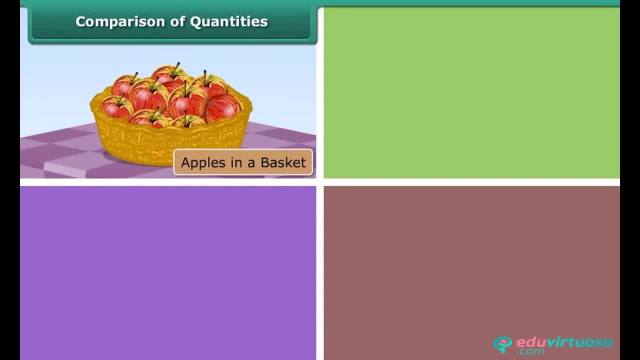 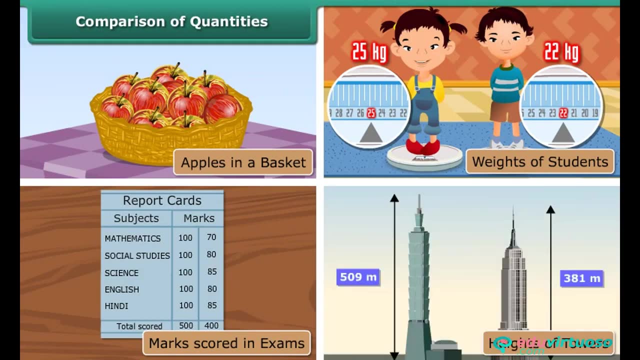 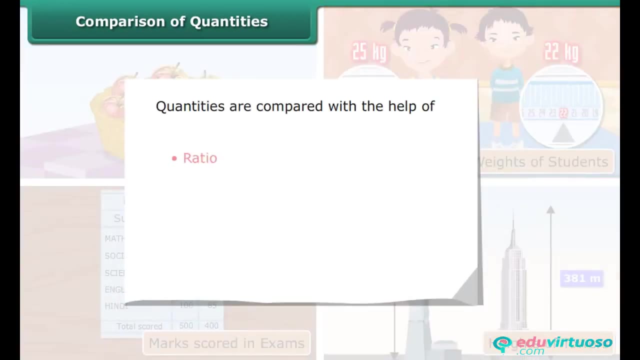 Comparison of quantities: Apple in a basket, weights of students, Marks scored in exams, Heights of towers, etc. Are all examples of quantities. Quantities are compared with the help of Ratio, proportion and unitary method. Let us look at these methods of comparison one by one. 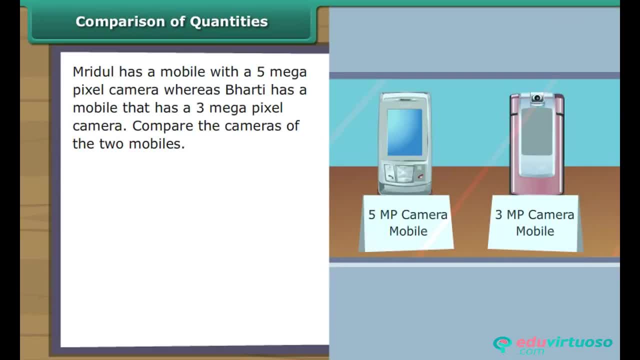 Ratio. Mridul has a mobile with a 5 megapixel camera, Whereas Bharti has a mobile that has a 3 megapixel camera. Bharti has a mobile that has a 3 megapixel camera. Lettuce compare the cameras of the 2 mobiles with the help of ratio. 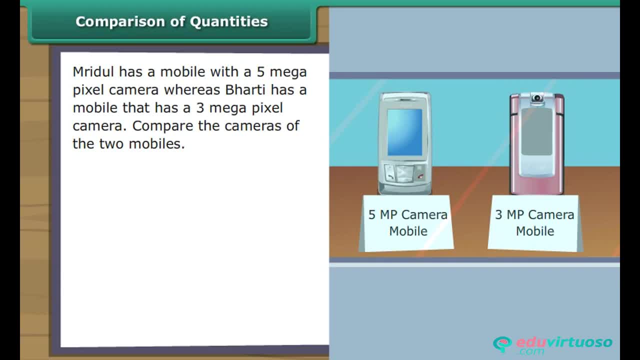 We express the ratio of the megapixels as 5 is to 3. It means That middle's camera is 5 by 3 times Superior to Bharti's camera. It also means that Bharti's camera is 3 x 5 times inferior to Music's camera. 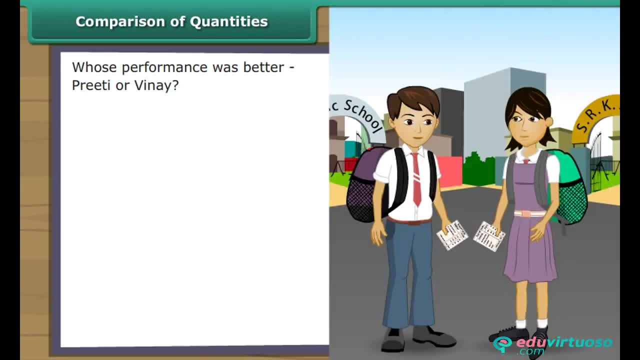 Proportion. Earlier in this lesson we had Preeti & Vinay argue that They're respective forces. their respective performances in the final exam were better. Let us sort the argument out with the help of proportion. Let us express the two total scores in the form of a ratio, as 400 is to 500. 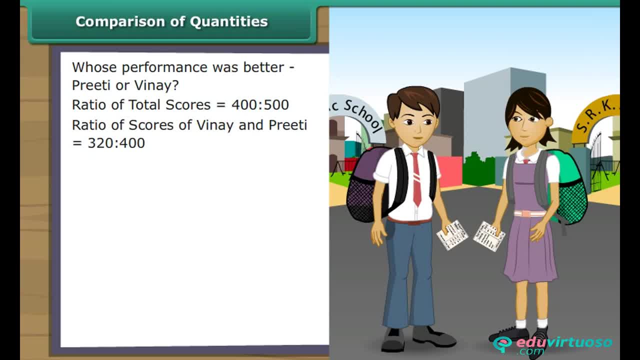 Now let us express the scores of Vinay and Preeti in the form of ratio, as 320 is to 400.. Reducing them to their lowest terms, we get: 400 is to 500 is equal to 400 divided by 500, which is 4 divided by 5.. 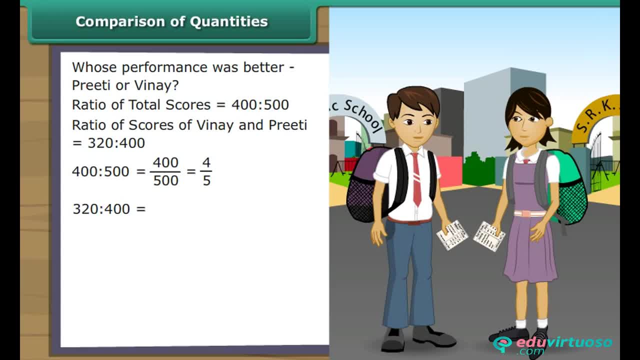 320 is to 400 is equal to 320 divided by 400, which equals 4 divided by 5.. It means the two ratios are in proportion. Therefore, both Preeti and Vinay were wrong. Both of them fared equally well in their final exams. 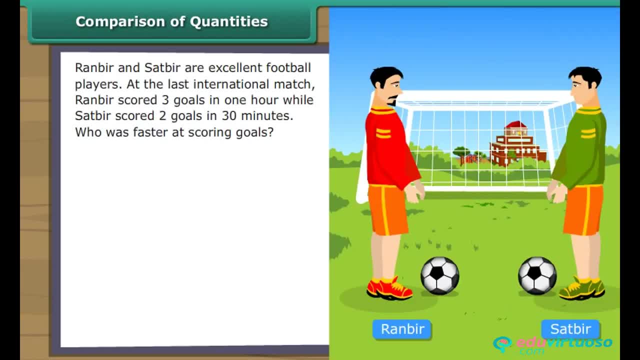 Unitary Method. Ranbir and Satbir are excellent football players. At the last international match, Ranbir scored 3 goals in 60 minutes, while Satbir scored 2 goals in 30 minutes. Who was faster at scoring goals? Let us solve the question with the help of Unitary Method. 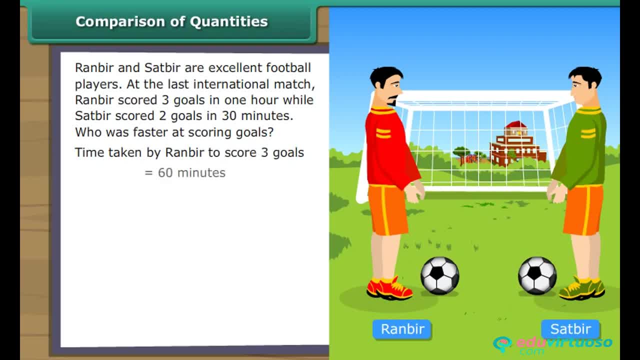 Time taken by Ranbir to score 3 goals is equal to 60 minutes. Time taken by Ranbir to score 1 goal is equal to 60 minutes. 1 goal is equal to 60 divided by 3, which equals 20 minutes. 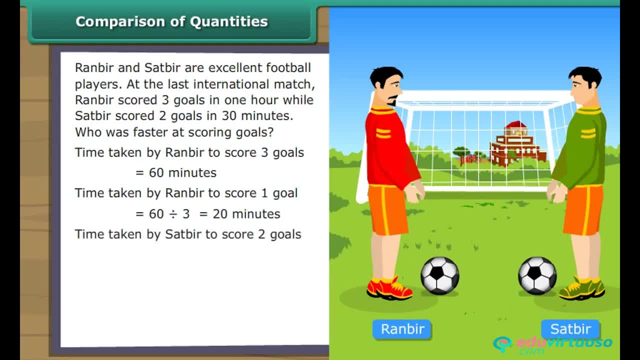 Time taken by Satbir to score 2 goals is equal to 30 minutes. Time taken by Satbir to score 1 goal is equal to 30 upon 2, which equals 15 minutes. Therefore, Satbir was faster at scoring goals. 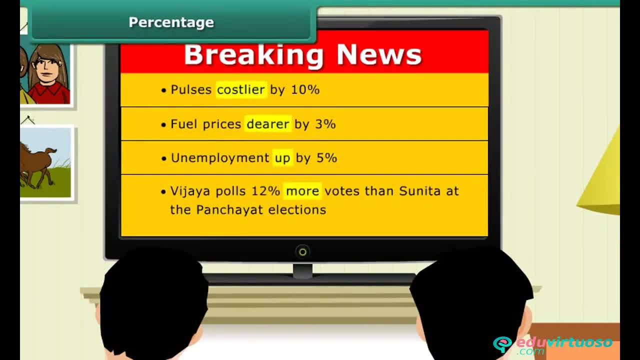 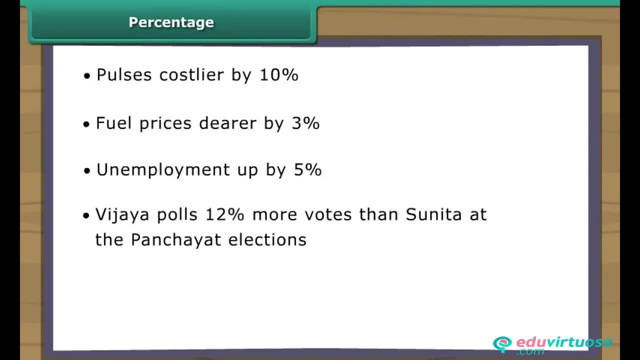 Percentage. Look at these new headlines: Pulse is costlier by 30 minutes. Pulse is costlier by 10%. Fuel price is dearer by 3%. Unemployment up by 5%. Vijaya polls: 12%. more votes than Sunita at the Panchayat elections. 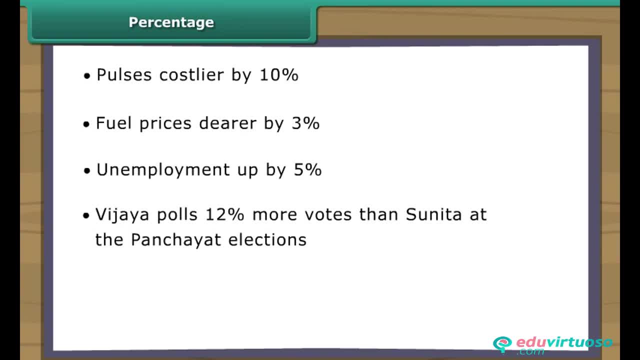 One common element in all these headlines is that they all indicate comparison of quantities. Another element common in them is the use of percentage symbol. The symbol denotes percentage. The term percentage literally translates to percentage. It divides despite weight. Москвit means numbers. 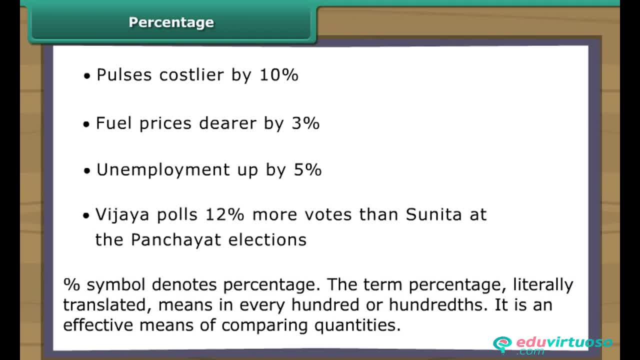 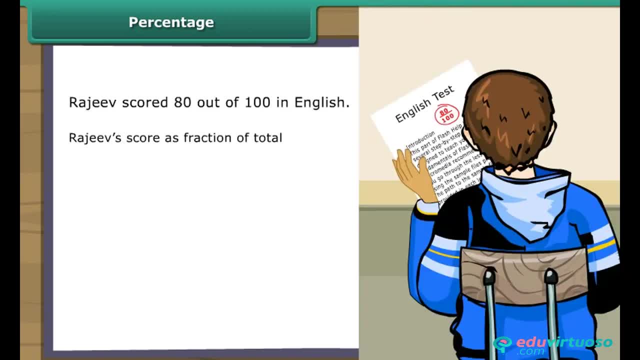 With numbers, you just divide them differently. So the number green means numbers. Rajiv scored 80 out of 100. in English His score can be expressed as A fraction of the total is 80 by 100.. The number fields is the size of the city. 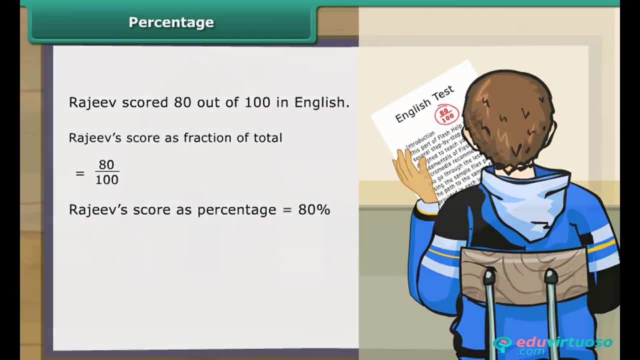 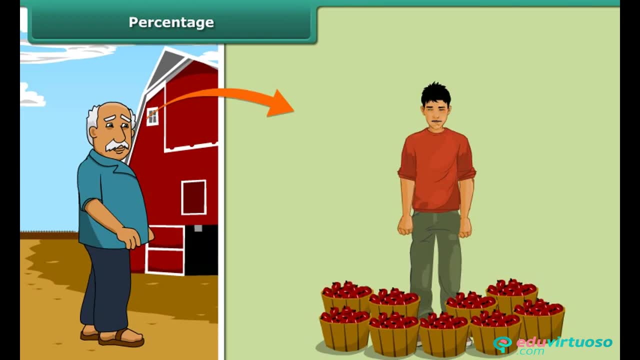 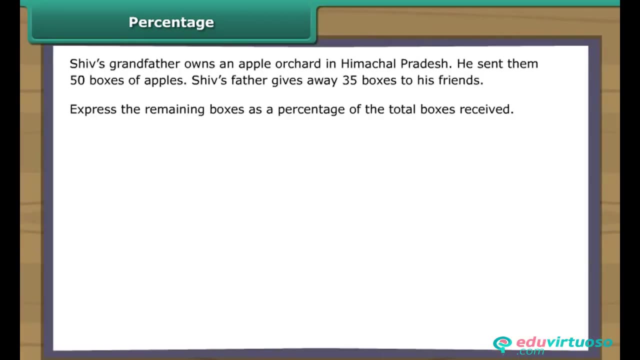 An average square times. Jum Sagarip P gebruvconomic away. 30TH means Shif's grandfather got an applegyard in Himachal Pradesh. He sends 50 boxes of apples, friends. let us express the remaining boxes as a percentage of the total boxes received. 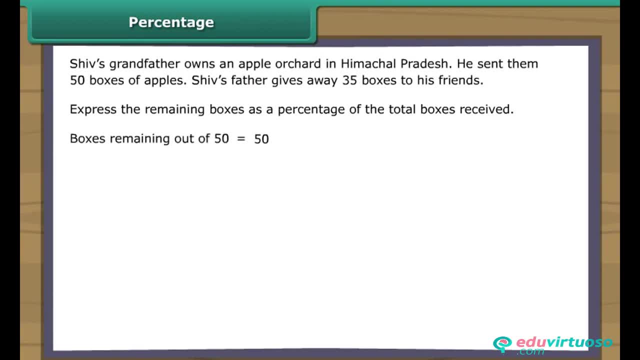 boxes remaining out of 50 is equal to 50 minus 35, which equals 15.. boxes remaining as a fraction of total boxes received equals 15 upon 50.. convert the denominator into 100. 15 upon 50 equals 15 into 2 upon 50, into 2, which equals 30 upon 100, which is equal to 30. 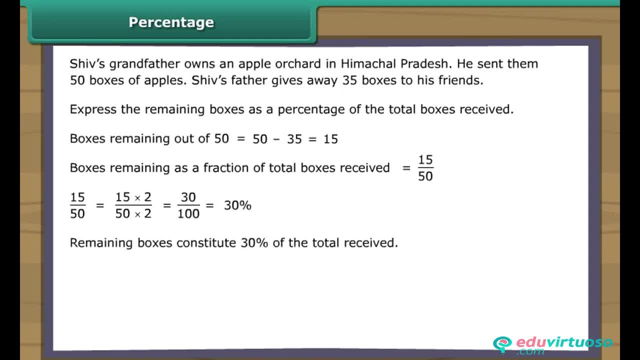 remaining boxes constitute 30 percent of the total received. let us attempt the same question with the help of the unitary method. boxes remaining out of 50 is equal to 15.. boxes remaining out of 100 is equal to 15, upon 50 into 100. 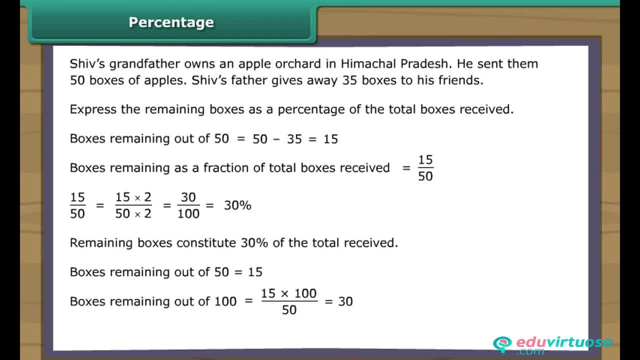 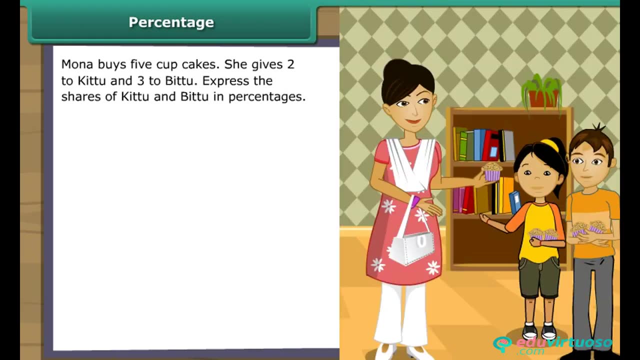 which equals 30. therefore, 30 percent of the total boxes received from shift's grandfather are with shift's family. both the methods yield the same answer. mona buys five cupcakes. she gives two to kittu and three to bittu. express the shares of kittu. 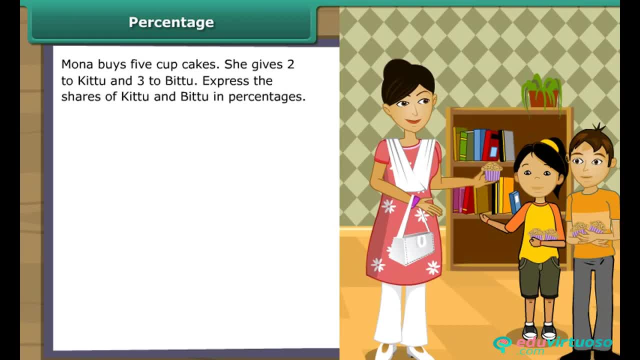 and bittu in percentages. number of cupcakes kittu gets out of a total of five is equal to two. number of cupcakes kittu gets out of a total of hundred is equal to two upon five into hundred, which is equal to forty percent. number of cupcakes bittu gets out of a total of five is equal to three. 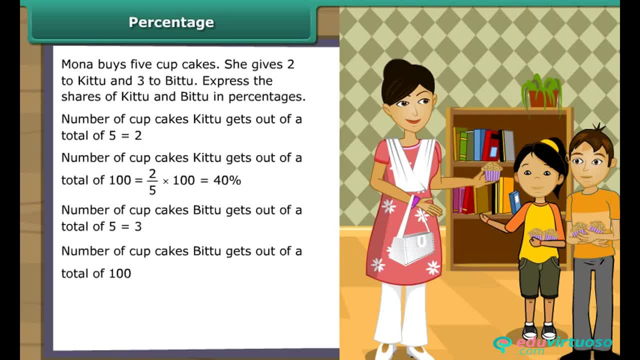 number of cupcakes bittu gets out of a total of hundred is equal to three upon five into hundred is equal to sixty percent. sum of percentages is equal to hundred percent. hundred percent represents the whole. in other words, it is the self-assessment. read the question carefully and select the correct. 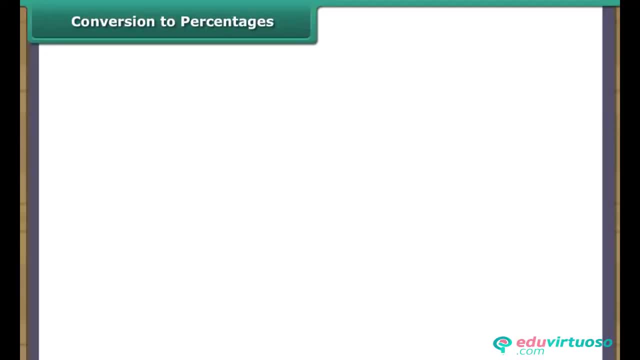 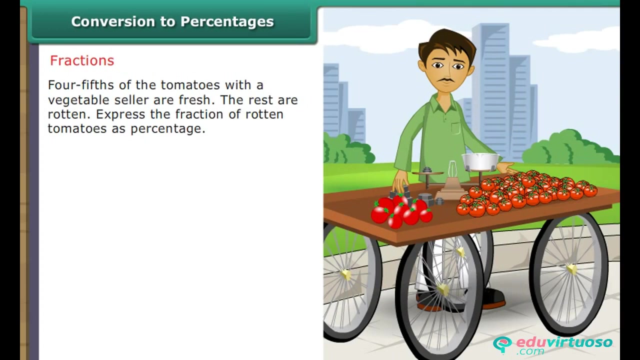 option: conversion to percentages. we have learned to express numbers as percentages. let us now learn to convert fractions, decimals and ratios into percentages. fractions: four-fifths of the tomatoes with a vegetable cellar are fresh. the rest are rotten. express the fraction of rotten tomatoes as percentage fraction of total tomatoes that. 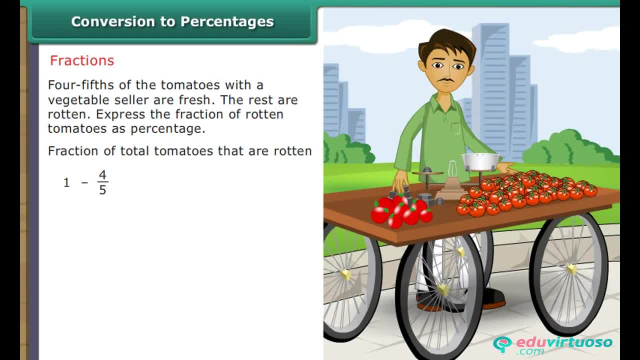 are rotten is equal to 1 minus 4 upon 5, which equals 1 upon 5. it means that 1 in every 5 tomatoes is rotten. number of rotten tomatoes in a total of 5 tomatoes is equal to 1. number of rotten tomatoes in a total of 100 tomatoes is equal to. 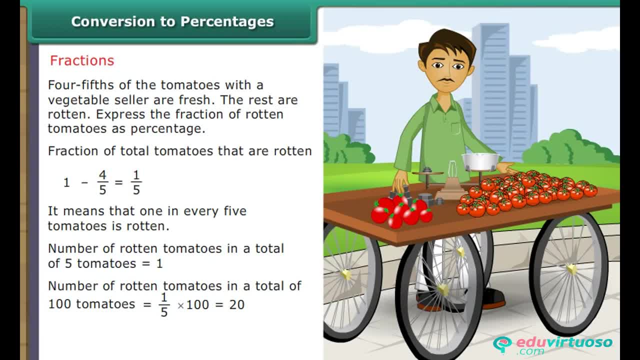 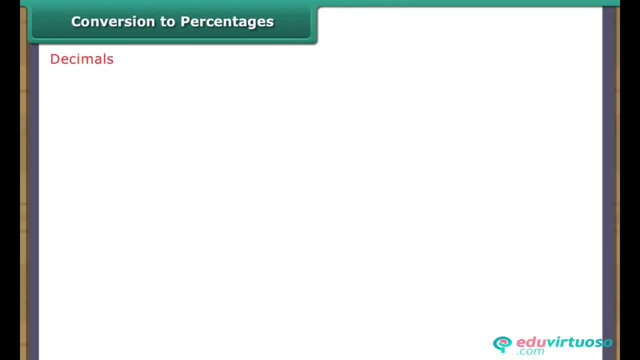 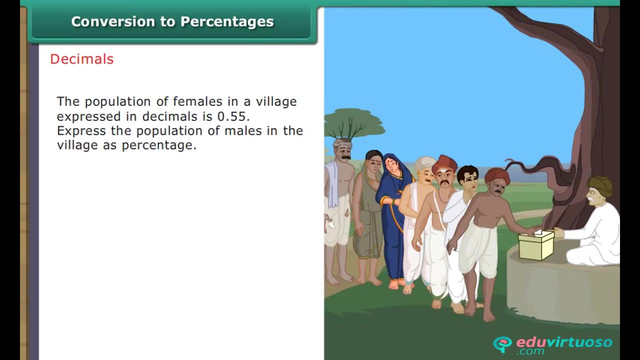 1 upon 5 into 100, which equals 20. 20 percent of the total tomatoes is rotten. decimals: the population of females in a village, expressed in decimals, is 0.55. express the population of males in the village as percentage population of females is equal to 0.55, which equals 55 upon 100, which is equal to 55. 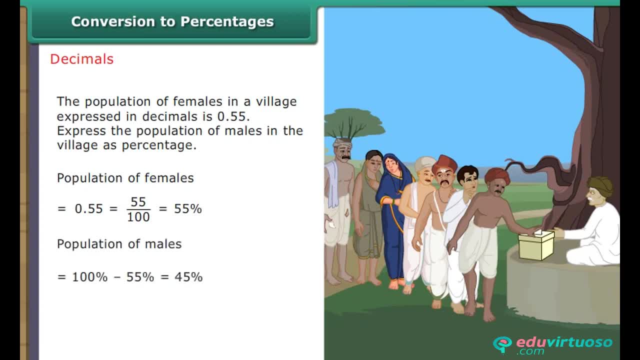 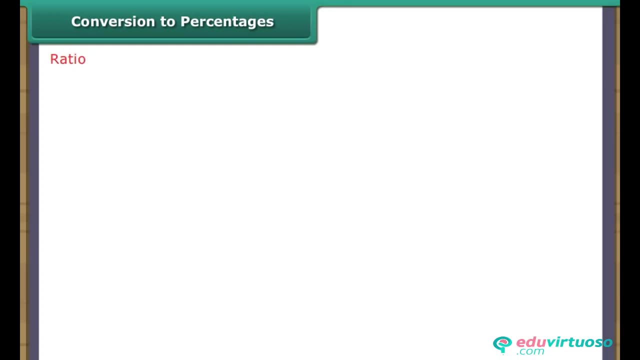 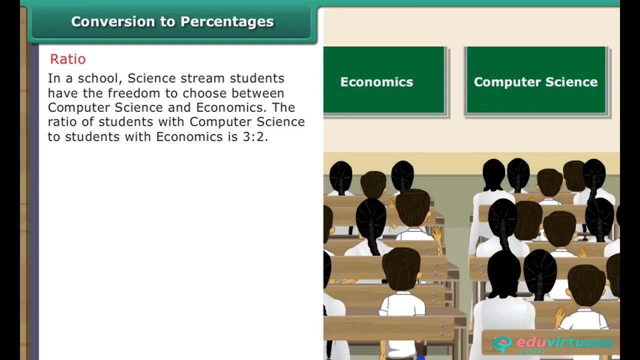 percent population of males is equal to 100 percent minus 55 percent, which is equal to 45 percent. males in the village form 45 percent of the total population ratios in a school. Vogt equals 5. Can continuing science be a five world or a five world science? 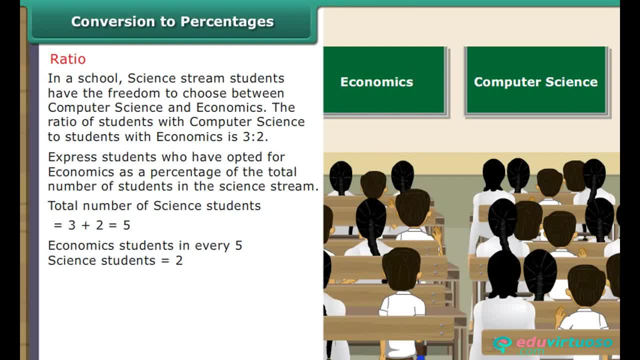 can continuing science be a five world or one world science? can continuing science be or fiveantic science? how do we improve the science ofни plus science such that 0.35 so 0 and 2, 0.50 is equal elastic Economic students in every 5 science students is equal to 2.. 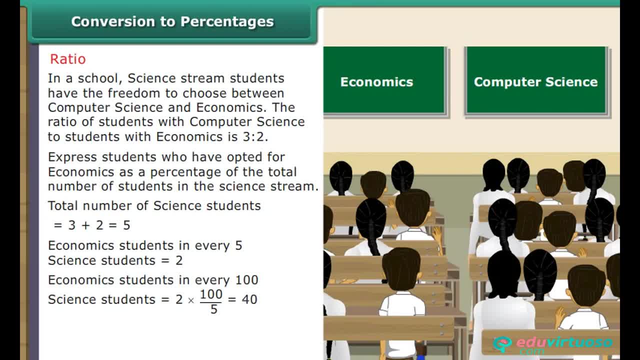 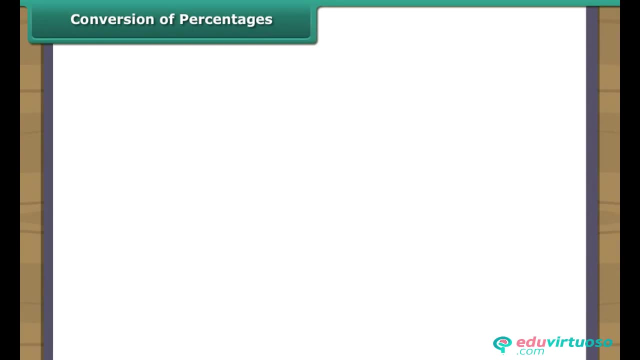 Economic students in every 100 science students is equal to 2 upon 5 into 100, which equals 40.. 40% of the science students have opted for economics. Conversion of percentages. We can now express numbers, fractions, decimals and ratios as percentages. 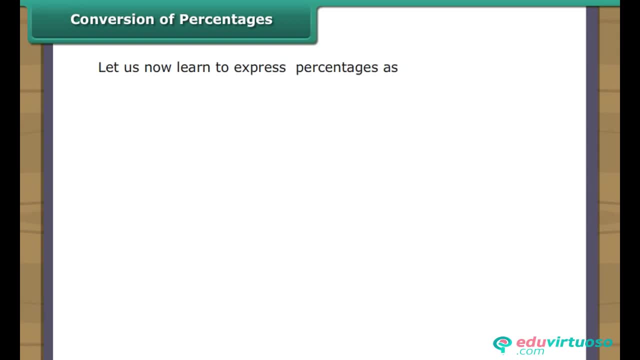 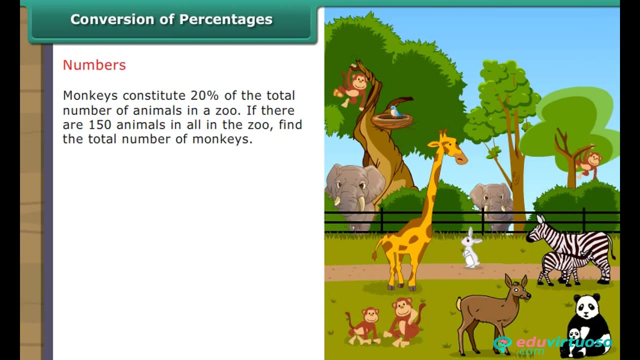 Let us now learn to express percentages as numbers, fractions, decimals and ratios. Numbers: Monkeys constitute 20% of the total number of animals in a zoo. If there are 150 animals in all in the zoo, find the total number of monkeys. 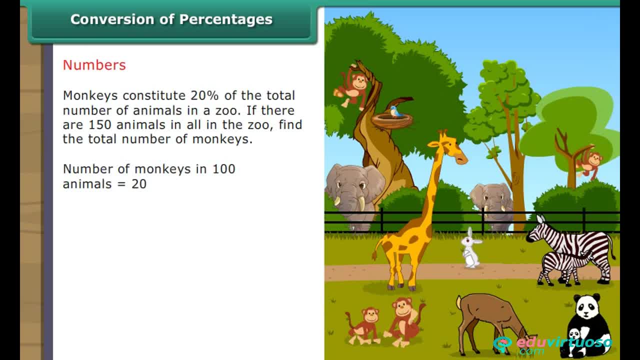 Number of monkeys in 100 animals is equal to 20.. Number of monkeys in 100 animals is equal to 20.. Number of monkeys in 150 animals is equal to 20 upon 100 into 150, which equals 30. There are 30 monkeys in the zoo. 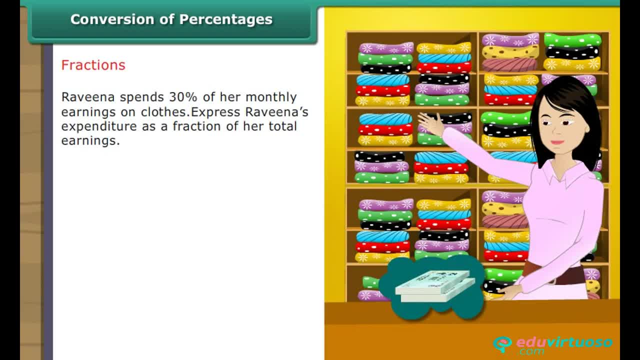 Fractions. Raveena spends 30% of her monthly earnings on clothes. Express Raveena's expenditure as a fraction of her total earnings. Amount spent by Raveena: out of every rupees 100, she earns rupees 30.. 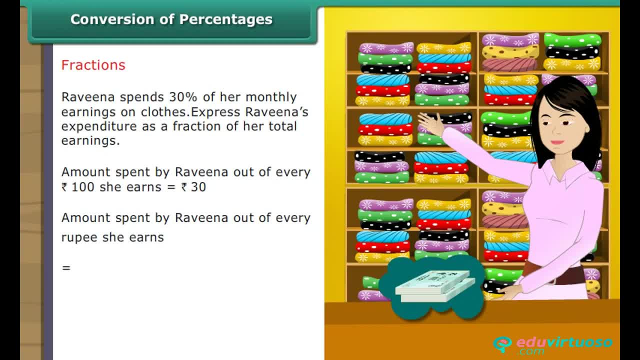 Amount spent by Raveena: out of every rupees 100, she earns rupees 30. Raveena out of every rupees she earns is equal to 30 upon 100, which equals 3 upon 10.. Raveena spends 3T of her earnings on clothes. 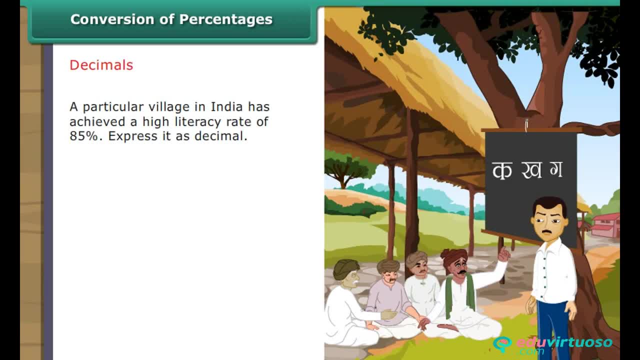 Decimals. A particular village in India has achieved a high literacy rate of 85 percent. Express it as decimal: Out of every hundred villages, 85 are literate Literates. as a fraction of 100 villages is equal to 85 upon 100, which equals 0.85. 85 percent expressed as decimal is 0.85 ratios 80. 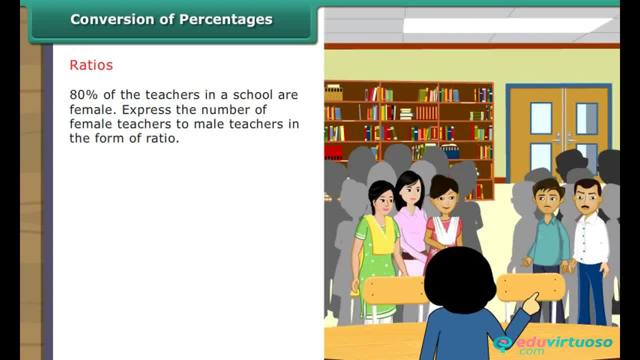 percent of the teachers in a school of female. express the number of female teachers to male teachers in the form of ratio. female teachers in every hundred teachers is equal to 80. male teachers in every hundred teachers is equal to hundred minus 80, which is equal to 20. the ratio of female teachers to male. 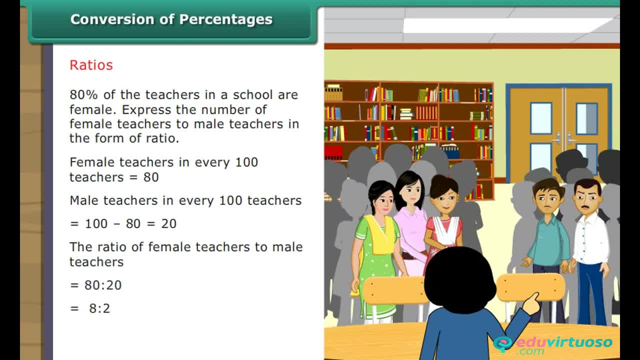 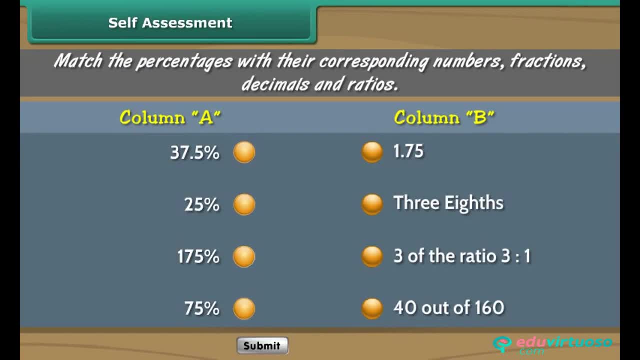 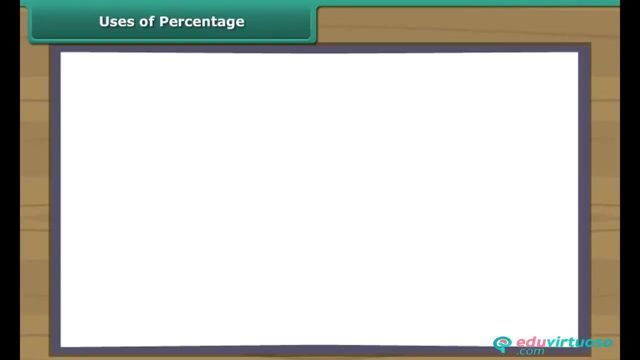 teachers. is equal to 80, is to 20, which is equal to 8, is to 2, which equals 4 is to 1. self-assessment. match the percentages with their corresponding numbers, fractions, decimals and ratios. you uses of percentage percentages are used to express many real-life situations. 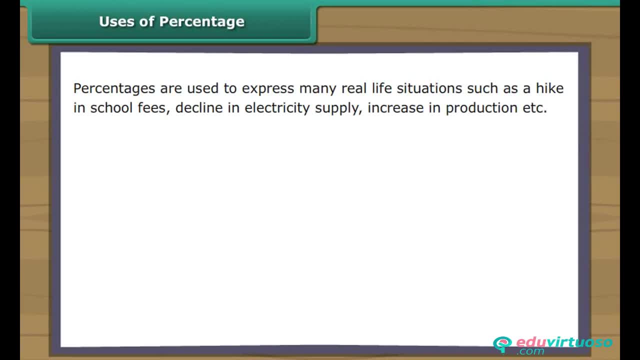 such as a hike in school fees, decline in electricity supply, increase in production, etc. we will now use the concept of percentage to represent increase or decrease, profit or loss and simple interest. increase, decrease, increase, decrease. percent is equal to increase. decrease upon original value into hundred. the price of petrol increases from rupees 50 to rupee sixty. 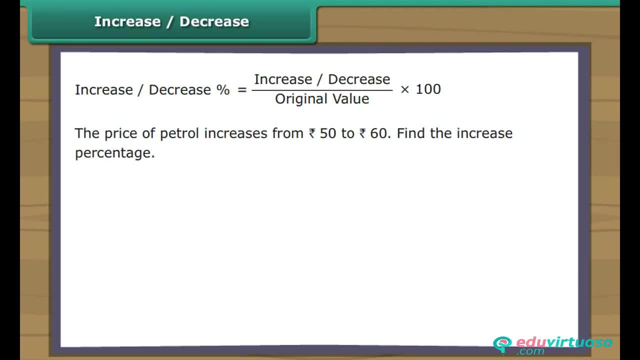 find the increase percent here. original price is rupees 50. increase in price is equal to new price minus original price, which is equal to 60 minus 50, which equals rupees 10. increase percent is equal to 10 into 100 upon 50, which is equal to 20 percent. so the fuel prices have increased by 20 percent profit. 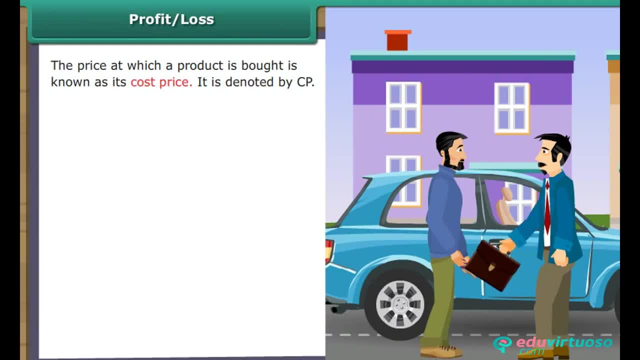 loss. the price at which a product is bought is known as its cost price. it is denoted by CP. the price at which a product is sold is known as its selling price. it is denoted by SP. if the selling price is more than the cost price, there is profit. profit is equal to SP minus CP. if the 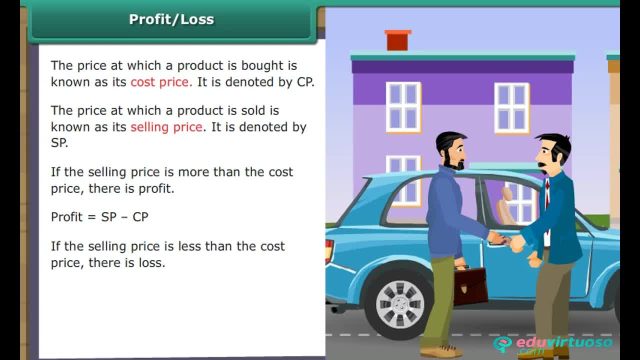 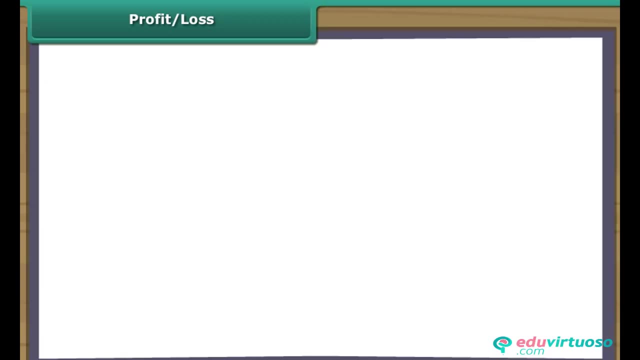 selling price is less than the cost price, there is loss. loss is equal to CP minus SP. profit or loss percent is equal to profit or loss upon CP into hundred. a shopkeeper buys an LCD TV for rupees 90,000 and sells it for rupees one. 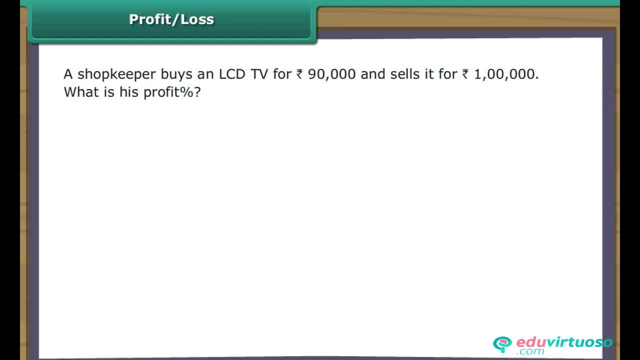 lakh. what is his profit percent? CP is equal to rupees ninety thousand. SP is its object. Benefit is equal to rupees 1 lakh. Profit is equal to SP minus. CP is equal to 1 lakh minus 90,000, which is equal to 10,000.. Profit percentage is equal to 10,000 into 100 upon 90,000, which is 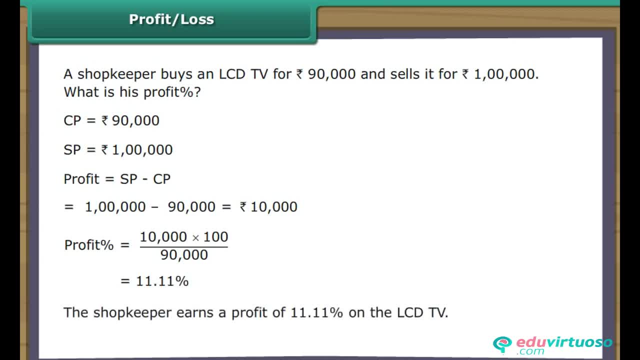 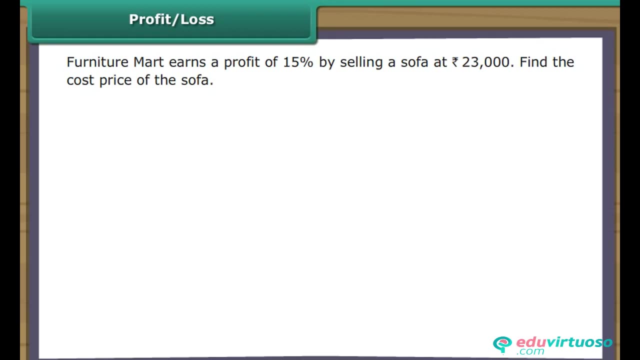 equal to 11.11 percent. The shopkeeper earns a profit of 11.11 percent on the LCD TV. Furniture mart earns a profit of 15 percent by selling a sofa at rupees 23,000.. Find the cost price of the sofa. Profit percentage is equal to SP minus CP upon CP into 100. 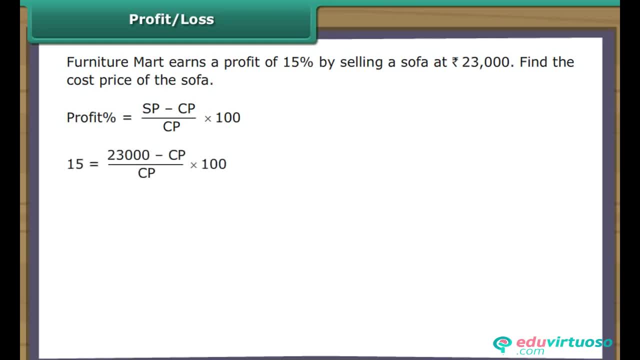 15 is equal to 15.11 percent. The shopkeeper earns a profit of 11.11 percent on the LCD TV. 15 CP is equal to 23,000 minus CP upon CP into 100.. 15 CP is equal to 23,000 minus CP into 100. 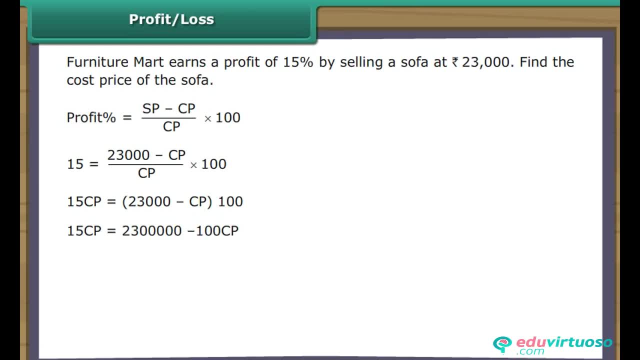 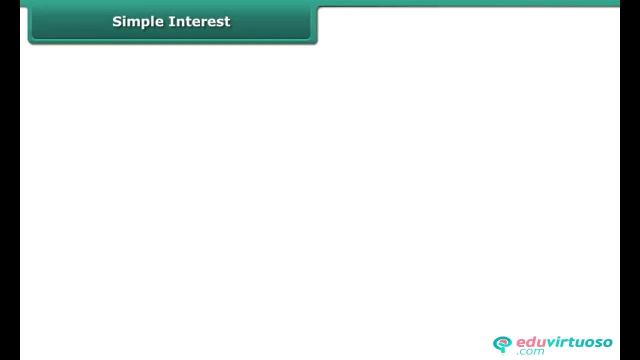 15 CP is equal to 23 lakh minus 100 CP, 115 CP is equal to 23 lakh. CP is equal to 23 lakh upon 115, which equals rupees 20,000.. The cost price of the sofa was rupees 20,000.. Simple interest: People deposit money in bank. 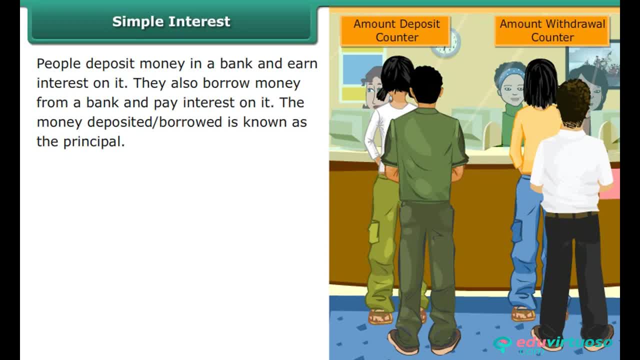 and earn interest on it. They also borrow money from a bank and pay interest on it. The money deposited or borrowed is known as the principal Interest payable on deposits and borrowings. is expressed as a percentage of the principal per year or annum, like 2 percent per annum. 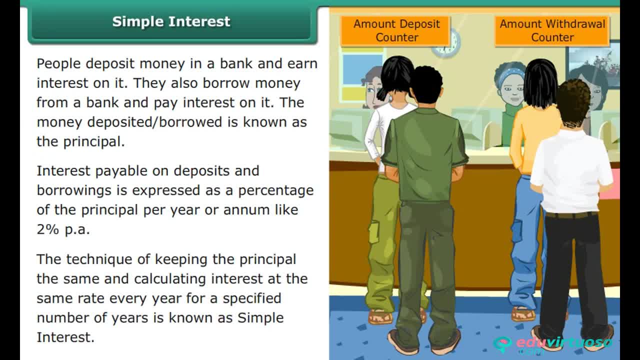 The court has a scientific classification to determine that the amount of interest each year, including the rate of interest you make per annum and deposit on months, plus Parker, The amount Principal Dun obeyed, since the attachment of the principal t and simple interest making of interest made a politics with simply interest, interest. 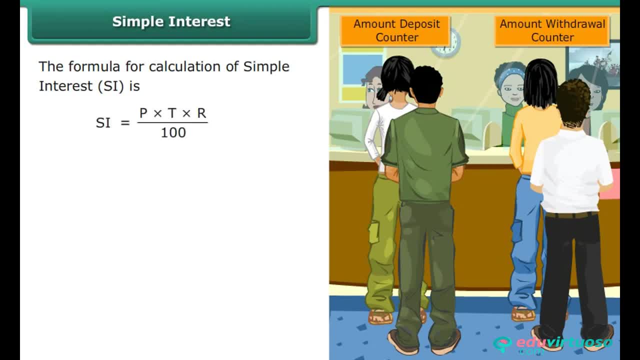 10 is the rate of interest. when the principal made a life here before, the bank gave him interest. then the principal gave him 40 days interest and public interest є is When the principal takes 100 currencies. This islo what is actually projecting. 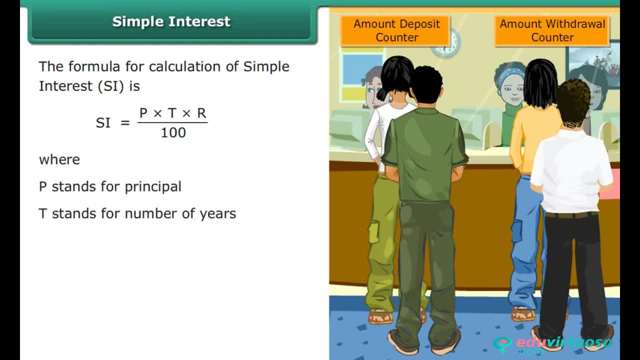 When processor took 60 coins, When $ is actually being Sver вообще $10.. Where can interest value if not $ means $? Yes, interest if the principal's interest, interest of the finance, is being with the principal, but not the principal's interest. savior does not belong. 2001'th cent on 2,000 dollars. 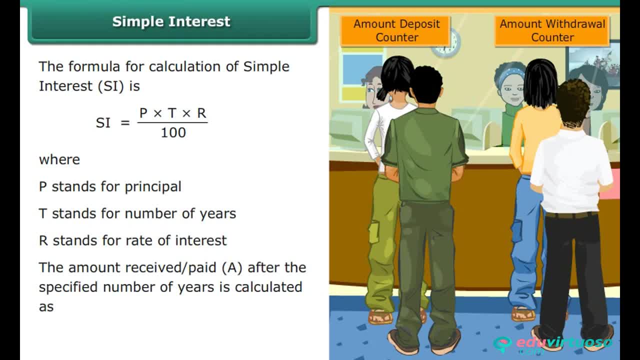 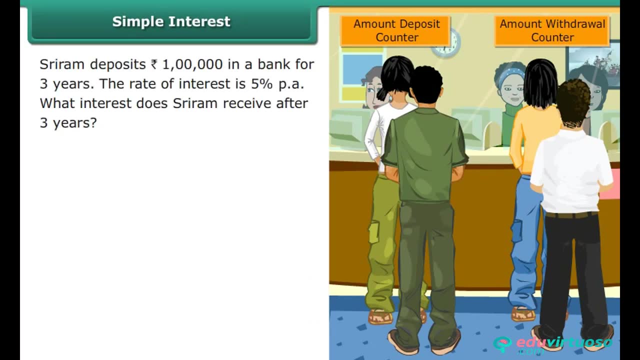 So if you want to do after, the specified number of years is calculated as a is equal to P plus SI. let's take a look on an example. serum deposits rupees 1 lakh in a bank for three years. the rate of interest is 5% per annum. what interest does Sri Ram? 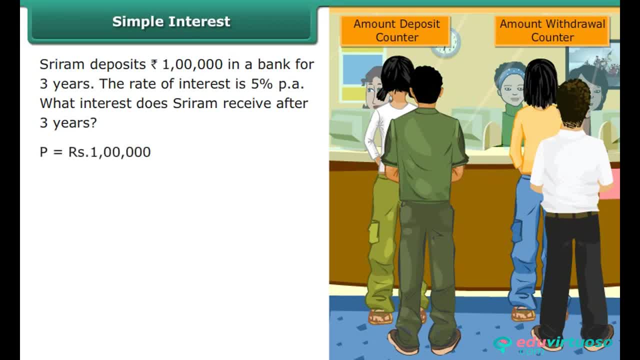 receive after three years. here principal is rupees. 1 lakh. time period is three years. rate on interest is 5%. now by substituting the values in the formula we get: SI is equal to 1 lakh into 3, into 5, whole upon 100, which equals rupees. 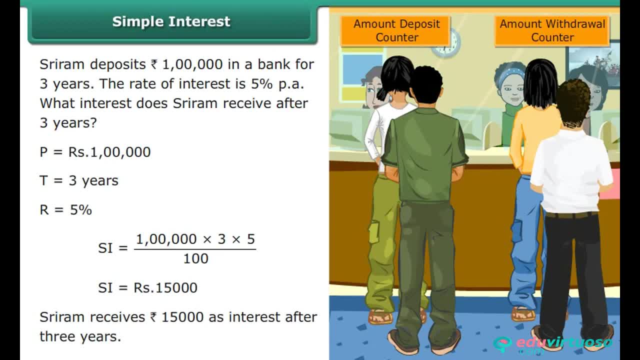 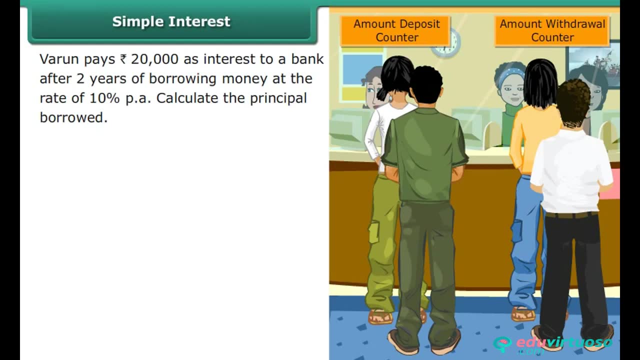 15,000. Sri Ram receives rupees 15,000 as interest after three years. now look at the next example in which we will calculate the principal. Varun pays rupees 20,000 as interest to a bank after two years of borrowing money at the rate of 10% per annum. calculate the principal borrowed here. 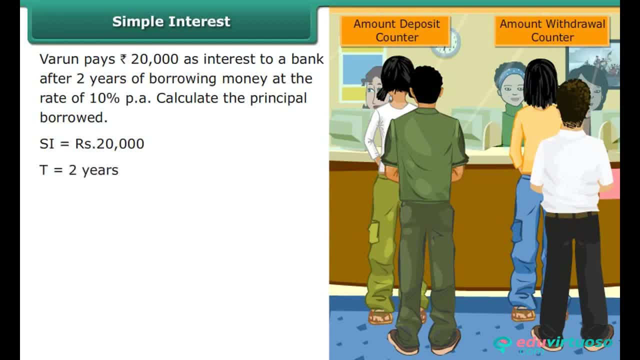 interest is rupees 20,000, time period is two years and rate of interest is 10%. now, by substituting the values in the formula, we get: 20,000 is equal to P into 2, into 10, whole upon 100. by calculating it, we get: 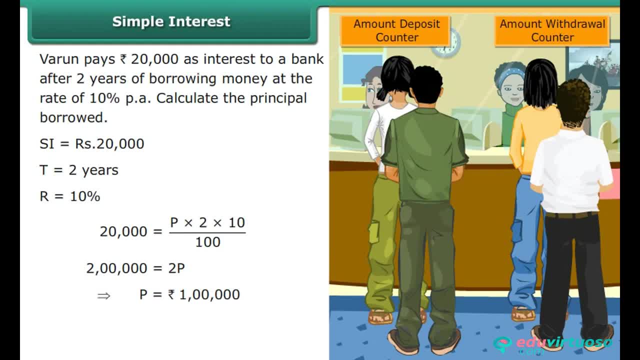 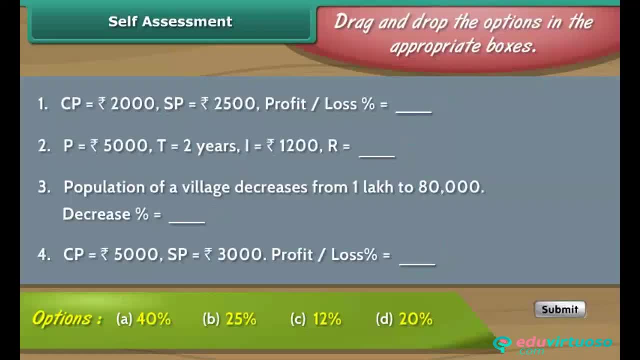 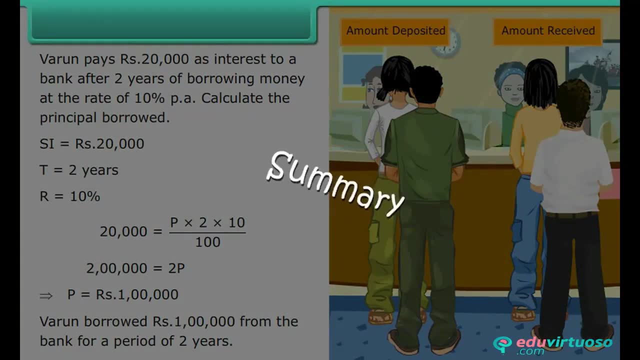 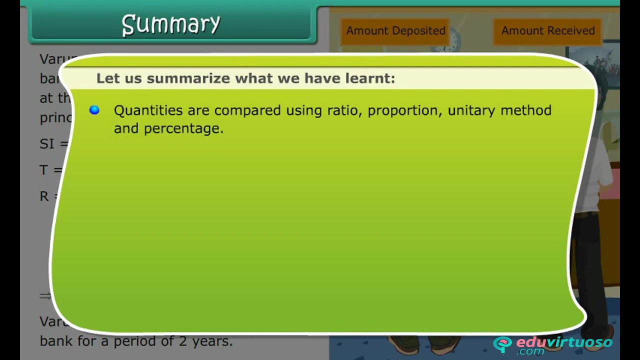 principal as rupees 1 lakh. Varun borrowed rupees 1 lakh for a period of two years. self-assessment- drag-and-drop the options in the appropriate boxes. summary. let us summarize what we have learned. quantities are compared using ratio, proportion, unitary method and percentage. 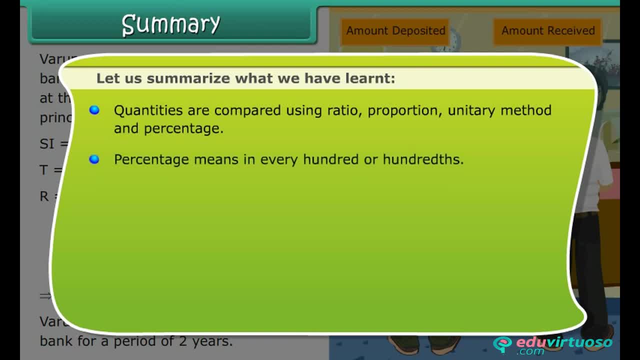 percentage means in every hundred or hundred. numbers, fractions, decimals and ratios can be expressed as percentages. percentages can be converted into numbers, fractions, decimals and ratios. the concept of percentage is used to compute profit or loss, percent, increase or decrease, percent and simple interest.